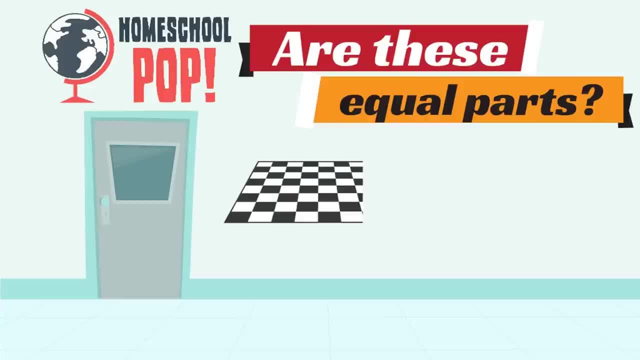 can make it into a game, right. okay, it's not like checkers, it's not like chess, you know. it's not like basketball, like soccer- okay, it's not like a game, game, game, okay. but it's still gonna be fun and we're gonna be able to see work with me here. okay, we're gonna be able to see if these pictures 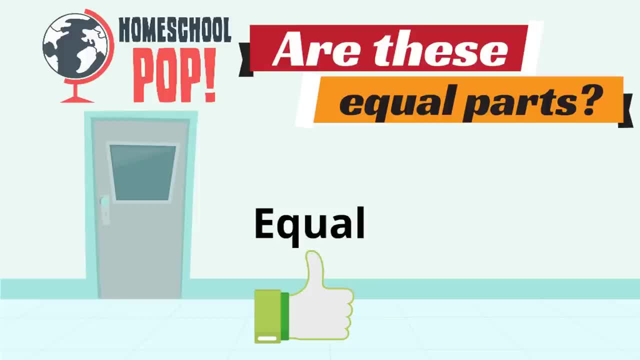 show equal parts or if these pictures show unequal parts. so here is our first picture. now we're gonna be looking to see if this picture shows equal parts, and this picture shows how many parts- two, good job. now. are these equal parts? yes, this picture shows two equal parts and we know they're equal. 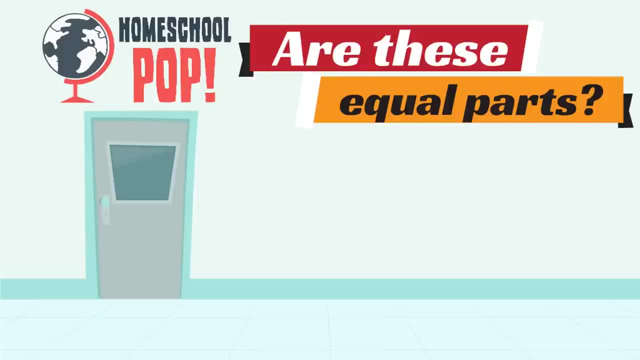 because they're the same size. now look at this one. this picture shows how many parts- yeah, three parts. now, are these equal parts? no, they're not equal parts. they're not equal parts because they're not all the same size. this picture does not show equal parts, great job. now let's give this picture a try. how many parts does? 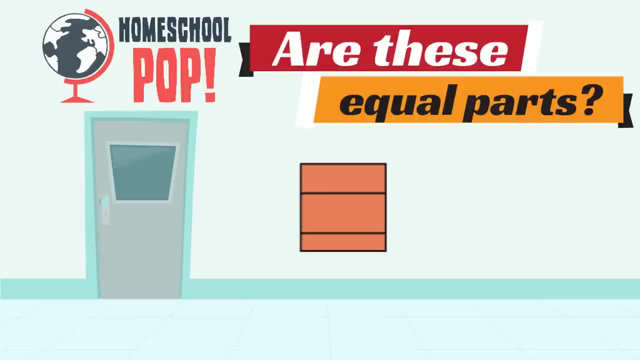 this picture show three. good job, and are these parts equal parts? no, they're not equal parts. can you imagine if you got that bottom part, if this, if this square was like a cake and you got that bottom part, that wouldn't be fair. why these are not equal parts. let's give this. 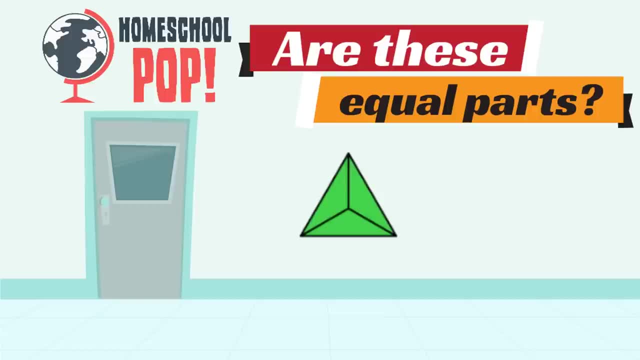 triangle picture a try. how many parts does this picture show? great job. three, and are these equal parts? Yes, they're equal parts because they are all the same size. Equal parts means each part is the same size. Great job. What about this picture? How many parts does this picture have? Be careful when. 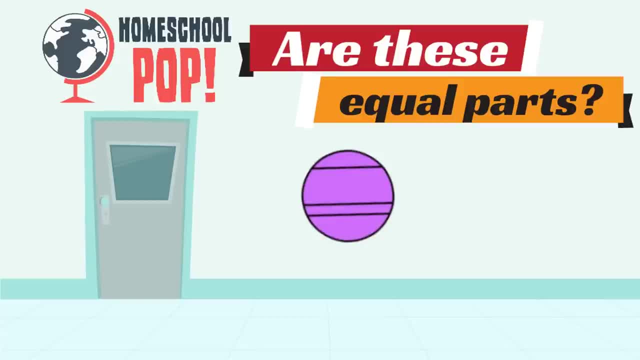 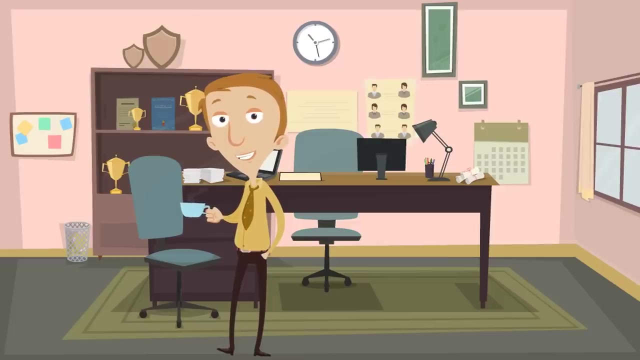 you count. It's a little bit tricky. This picture has four parts. Now are these equal parts? No, they're not equal parts. How do we know? Because they're not the same size. I don't know about you, but I feel pretty good about this equal parts. 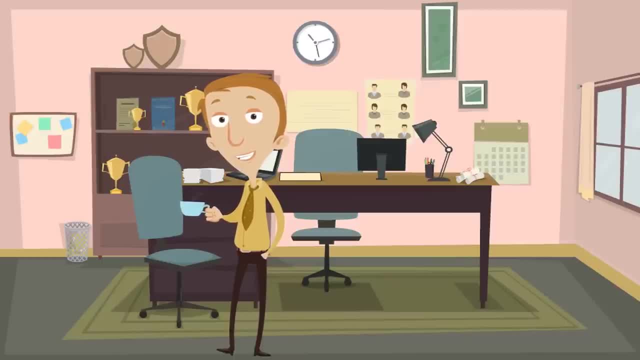 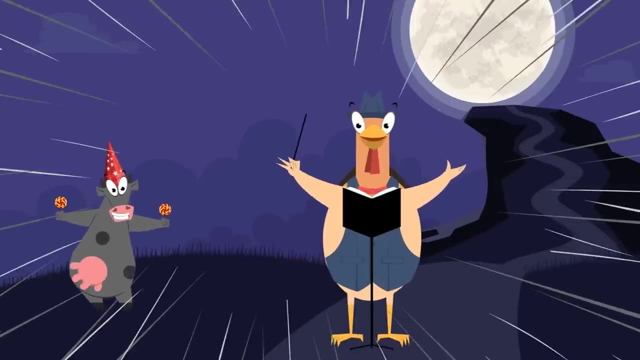 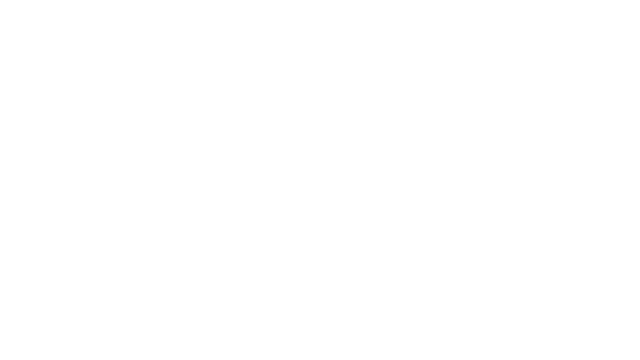 stuff. It just means that the parts are the same size. When they're the same size, that means they're equal. That's pretty cool. Let's keep going No with the game, the equal parts game. why would there be a turkey and a dancing cow? 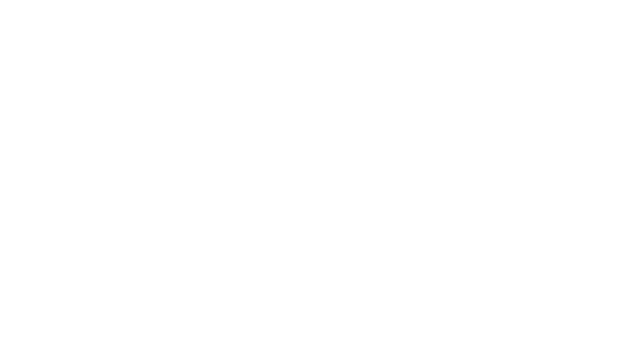 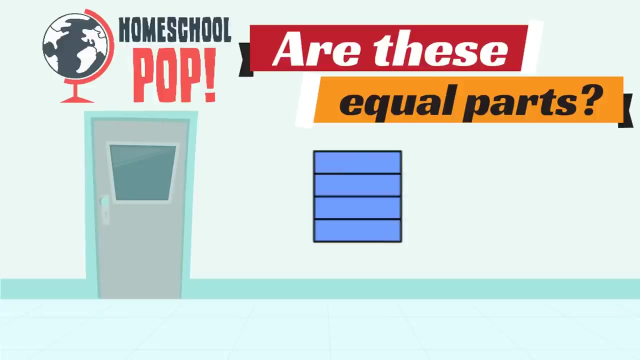 We're doing the equal parts thing here. okay, I meant let's get back to the game, please. Our next picture is this blue square. How many parts does this picture show? Great, It shows everything. Four parts. Now are these parts equal? 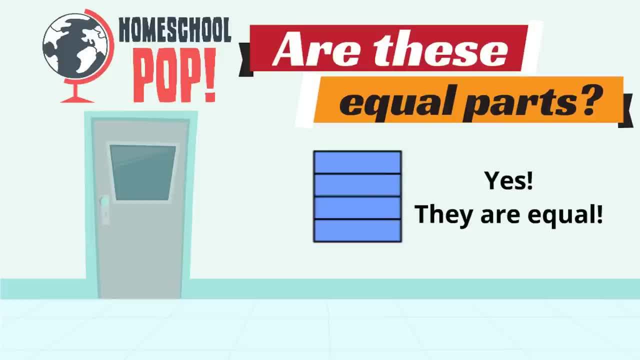 Are these equal parts? Yes, they're equal. How do we know? Well, these parts are equal because they're the same size. Check out this picture. It's a picture of a triangle. How many parts does this triangle have? Great Three. 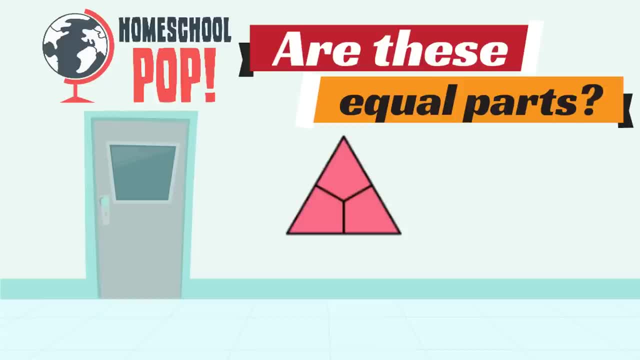 Are these equal parts? Look carefully. Yes, they're equal parts. How do we know? Well, these parts, the parts of the triangle, are all the same size. Well, I'm going to pick up the pizza now. I'm going to split it in four. 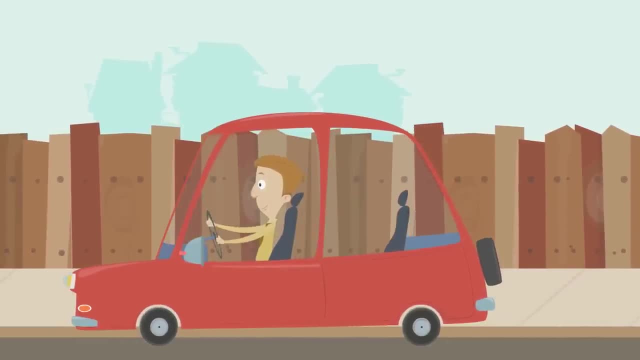 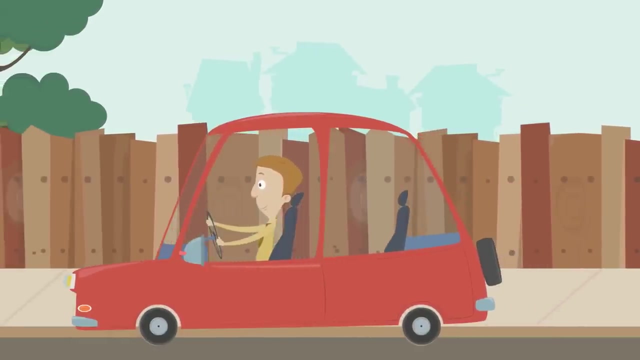 Four equal parts, Four equal parts. Four equal parts. Parts, Parts, Parts, Parts. Oh man, Oh, I should have rehearsed this song before I started singing. All right, Well, here we are. We're going to split the pizza in four equal parts.